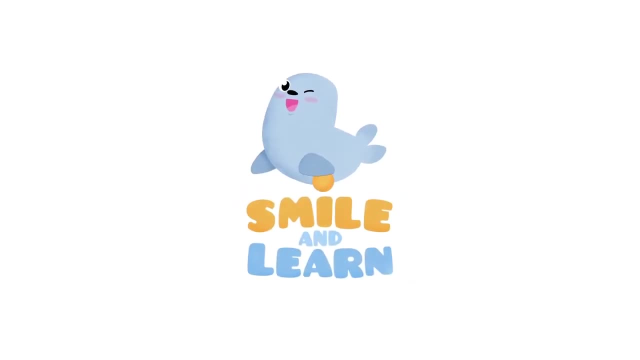 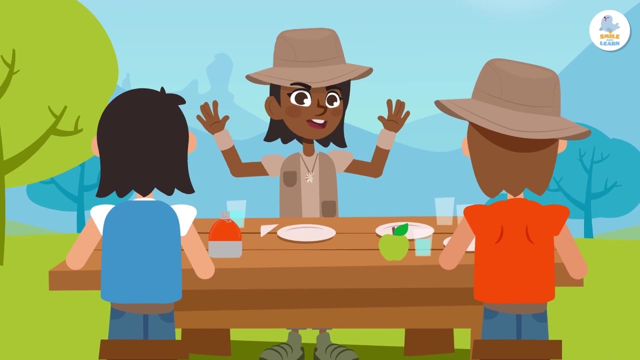 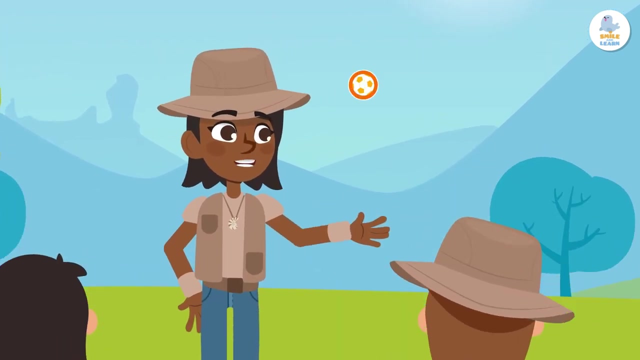 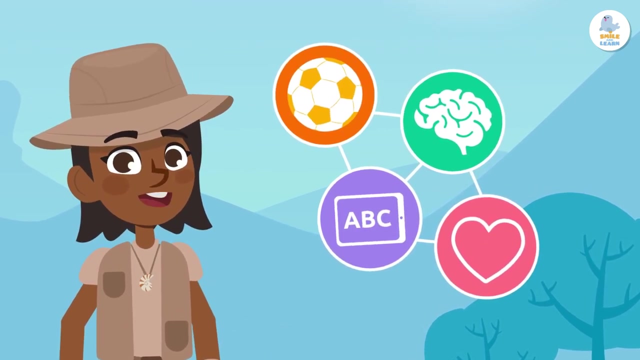 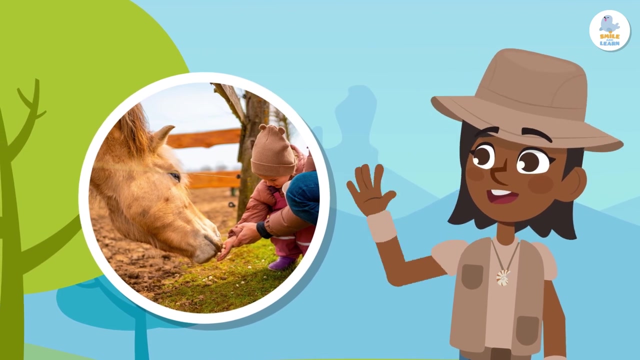 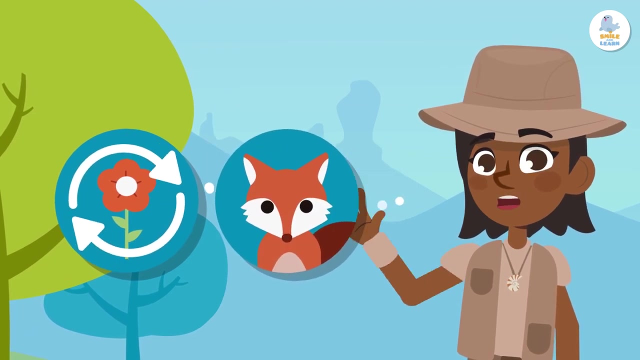 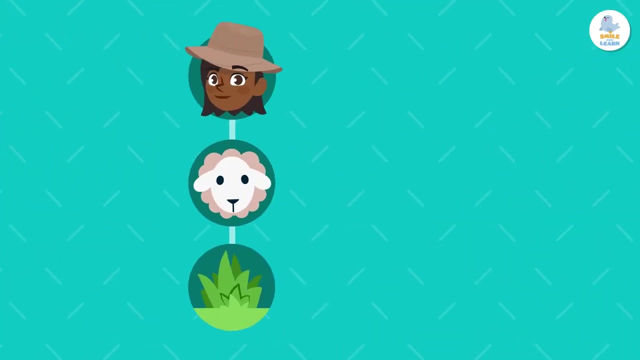 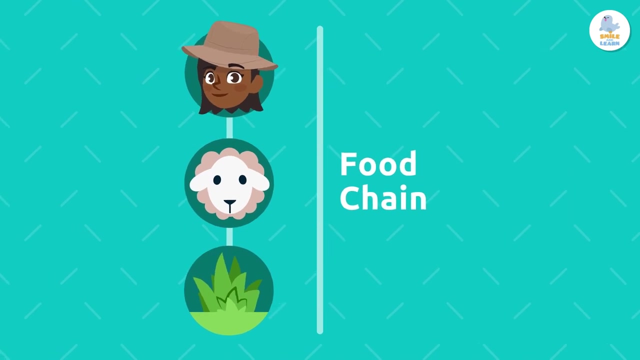 Smile and learn. Living things get energy from the food we eat. Some can produce their own food, while others get energy by eating plants or other animals. The way energy passes from one living thing to another is called a food chain. Have you ever heard of food chains? 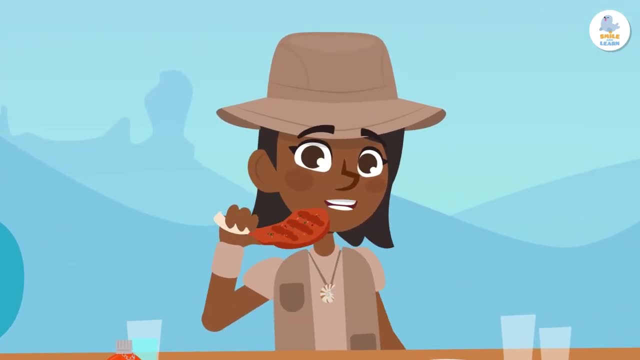 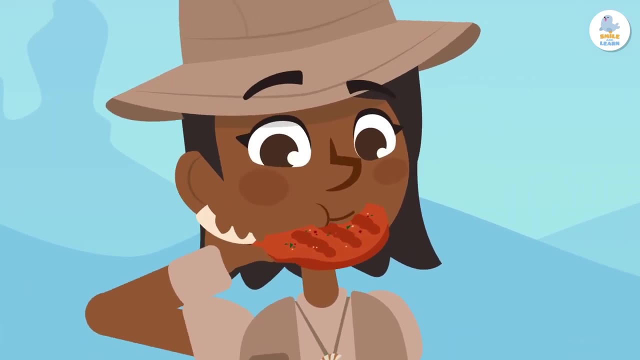 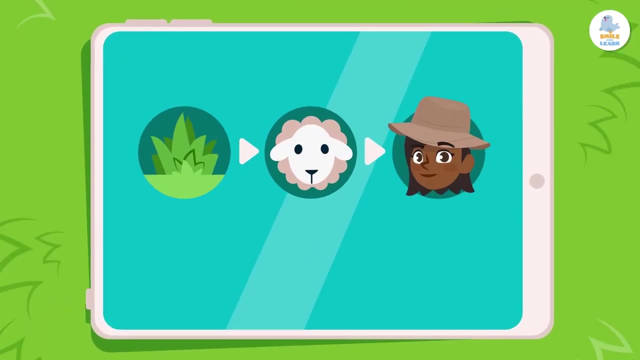 We are going to look at them now, But I'm getting a little hungry, So first I'm going to take a bite of my lamb chops: Mmm, yummy. So what is a food chain? anyways, It's a diagram that shows how living things are connected by what they eat. 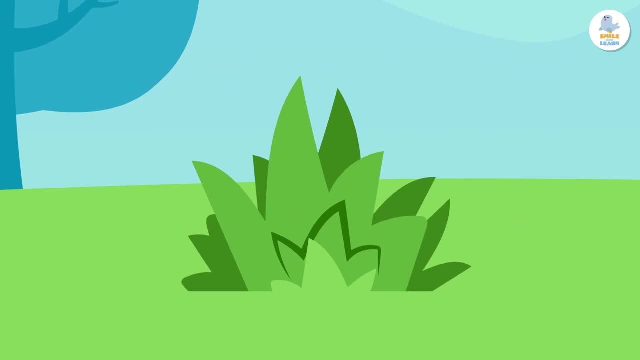 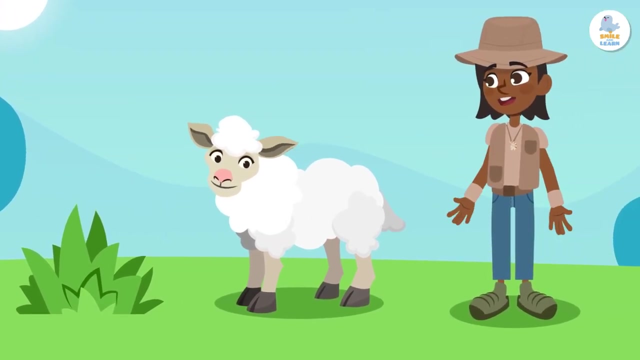 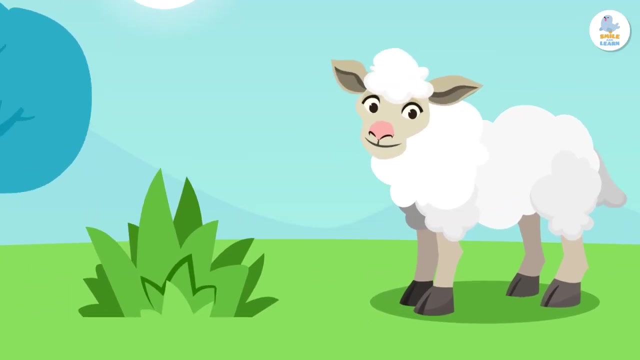 In other words, it tells us how plants and animals depend on each other. In fact, I'm part of a food chain right now. Let's see what the food chain looks like when I eat my lamb chops. At the first level, we have grass. 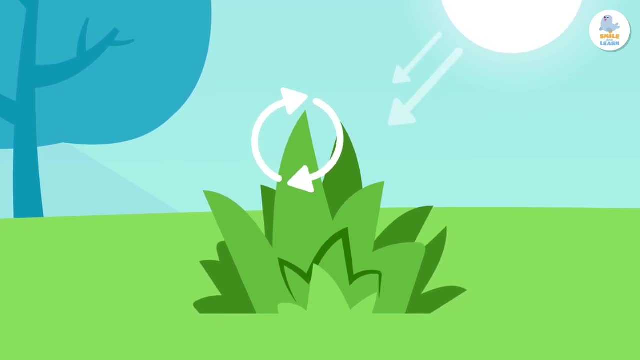 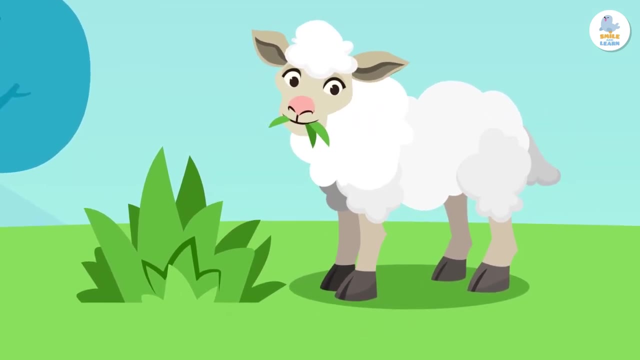 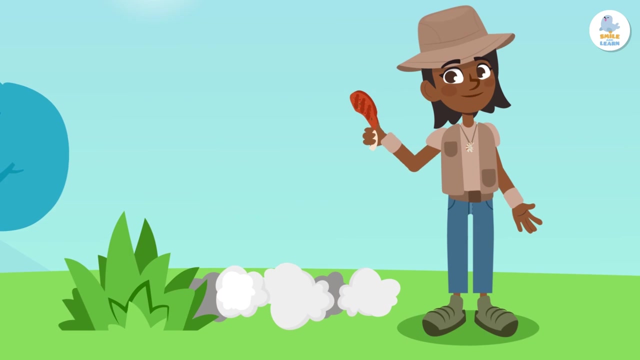 a plant that produces its own food through photosynthesis. Then, on the second level, we have a lamb which eats the grass. Finally, we have a tree. Finally, I'm on the last level, because I eat the meat from the lamb. 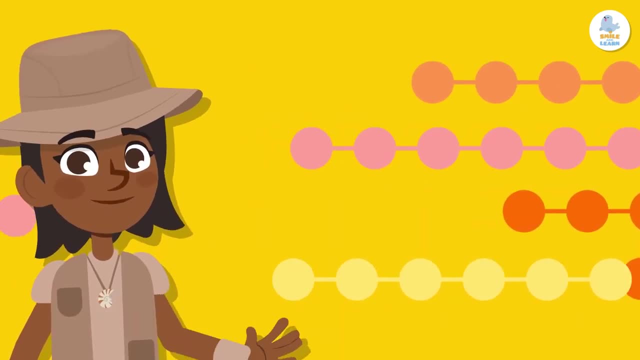 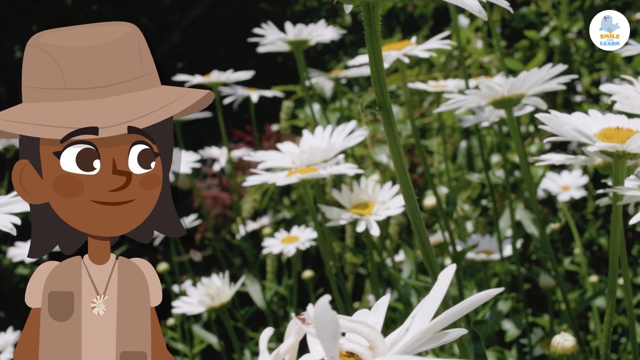 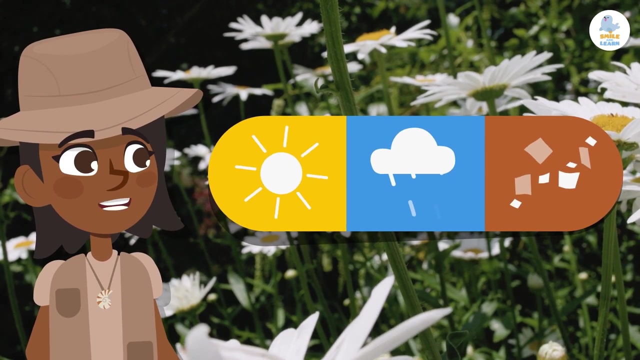 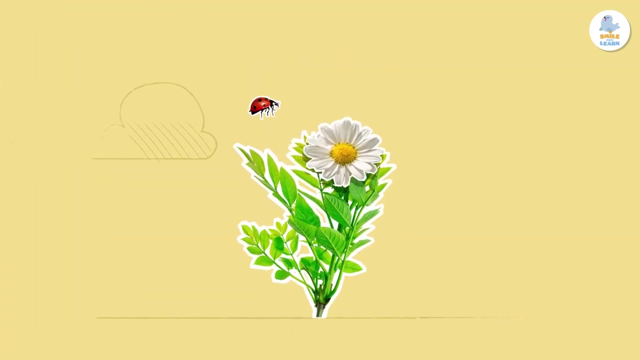 There are many food chains. Let's look at another, more complex example. Picture a beautiful flower. When the flower needs energy, it makes it from the sun, water and nutrients from the soil through photosynthesis. But along comes a very hungry ladybug and it eats the flower. 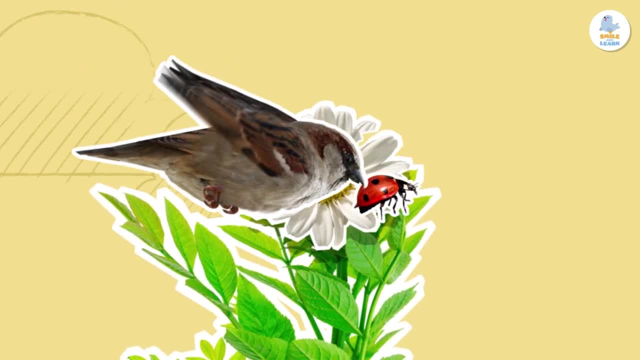 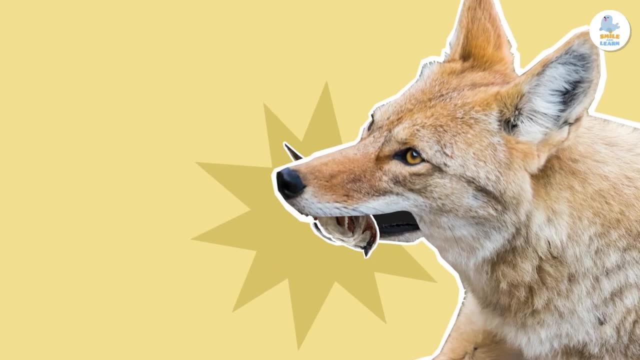 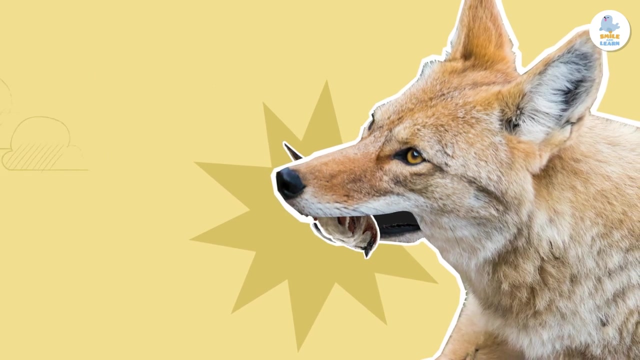 And then along comes a very, very hungry bird, so it eats the ladybug. But later a super hungry coyote comes along and eats the bird. Wow, Now this story gets a little sad, but it's something we can all do together. 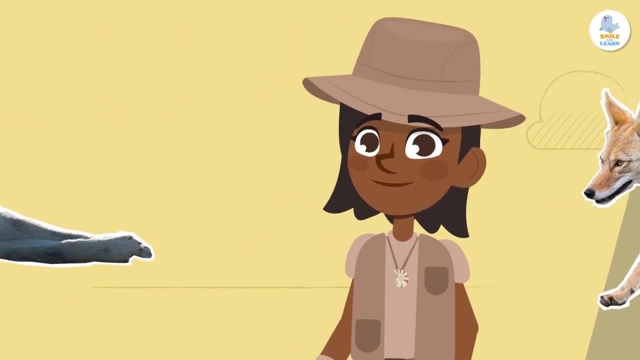 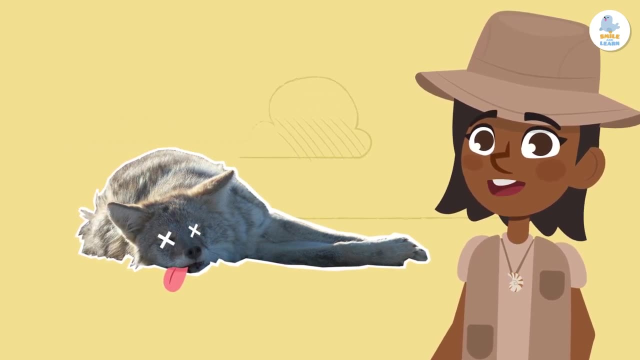 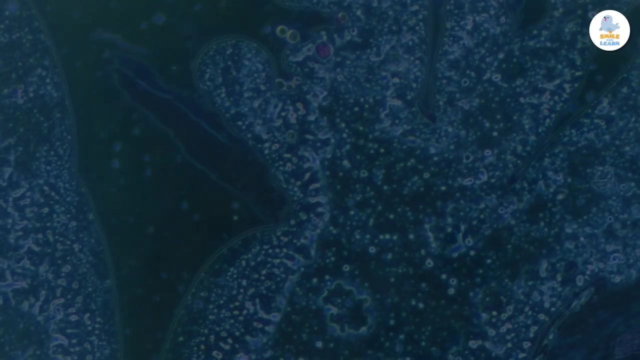 But it's something that happens to all living things. After a long and happy life, our coyote dies, But don't worry, This is when things get interesting. Now it's time for the bacteria and fungi to do their job. We can't see them, but they're everywhere. 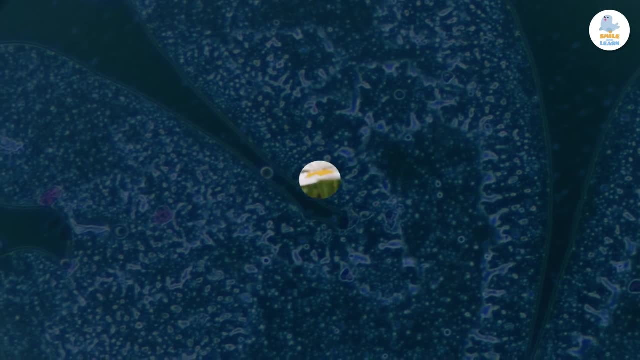 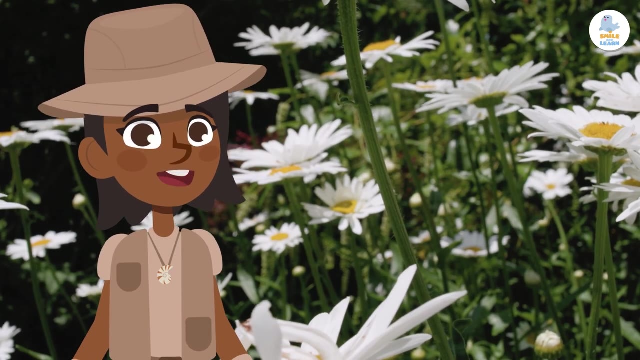 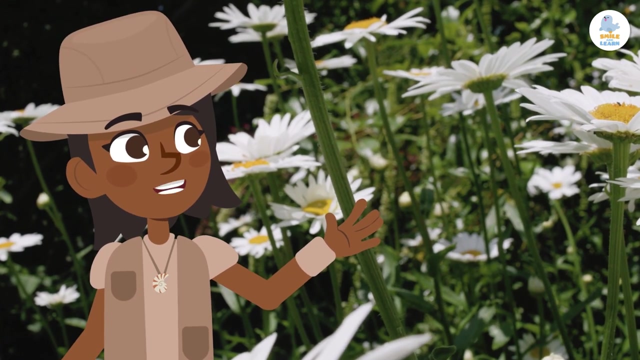 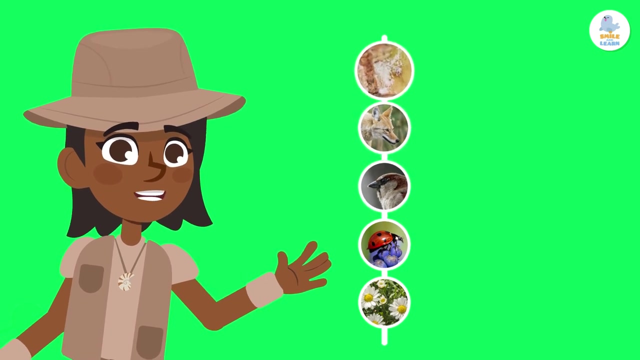 They will eat the coyote's body. When they do so, they turn the coyote into nutrients that the plants can use to make their own food. Amazing right, And so the food chain starts again. As you can see, food chains have different levels. 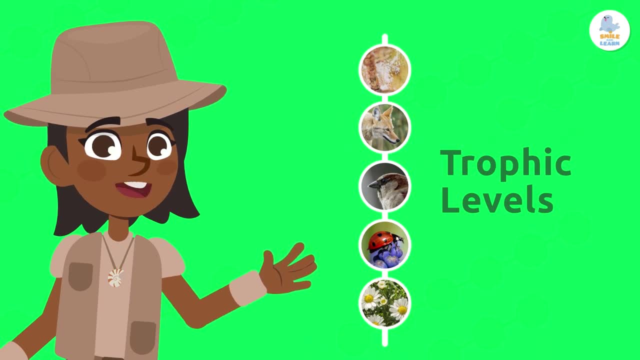 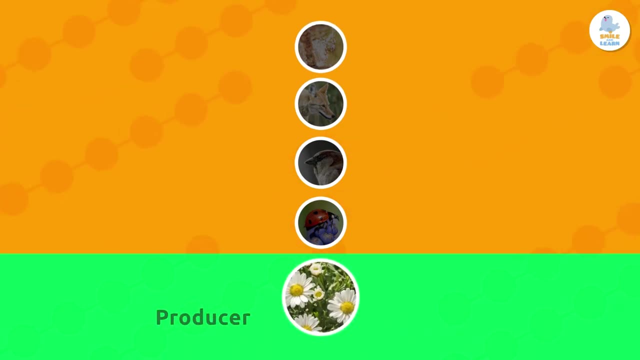 which we call trophic levels. Let's learn about them. Food chains can start with an autotrophic plant or producer that makes its own food. In the example from before, the flower is our producer, But, as we know, 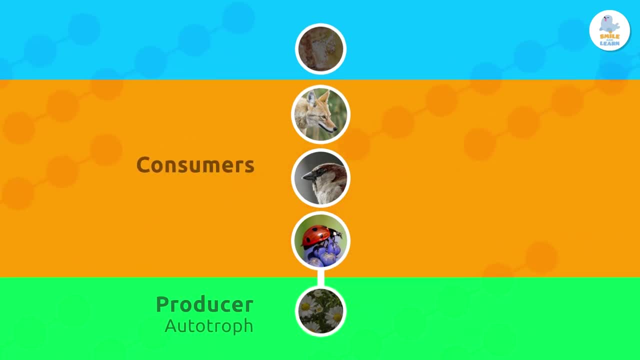 not all living things can produce their own food. These living beings are called heterotrophs, and they eat other living things to get energy. Animals that eat producers are called primary consumers. In this food chain, the ladybug is our primary consumer. 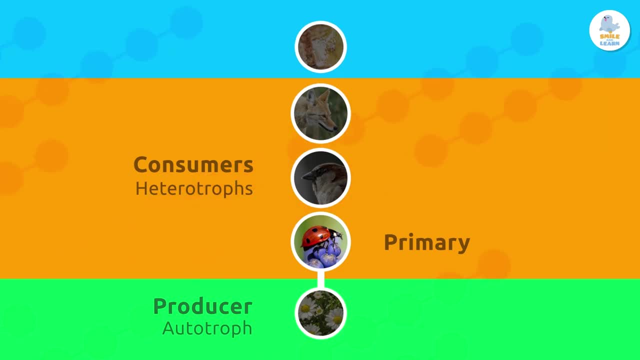 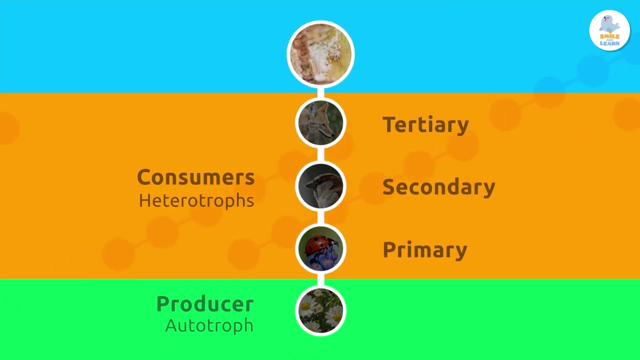 Next, there are animals that eat the primary consumers. These are called secondary consumers, like the bird in this food chain. Then animals that eat the secondary consumers are called tertiary consumers, like the coyote. Like the coyote in our example.